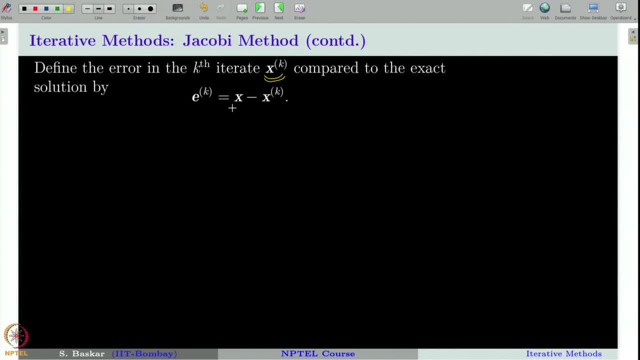 to the exact solution is defined as x minus xk and we use the notation ek to denote that quantity x minus xk. Well, if you recall, in the last class we have derived the expression for the iterative sequence of the Jacobi method and it is given by: xk plus 1 is equal to b. 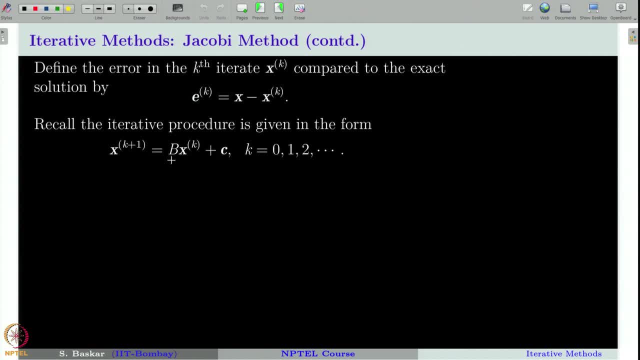 into xk plus c, where b is an n cross n matrix and c is a n dimensional vector. So we have derived the expression for this b. So we have derived the expression for this b for b and c in the last class and if you recall the same equation will also be satisfied by: 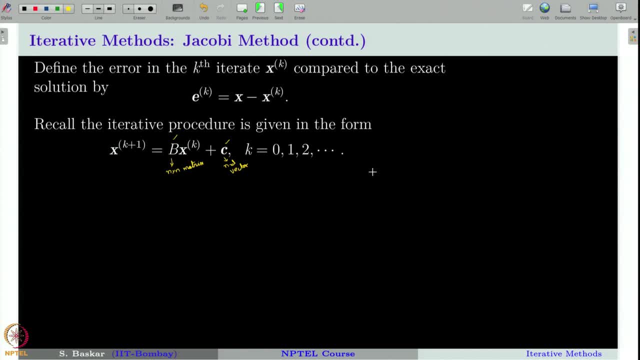 the exact solution of the linear system: A, x equal to b. That is, x also satisfies the equation x is equal to b, x plus c. Why? Because, simply, we have written A, x equal to b in this form. that is all. we did not do anything. we just rewritten this system in this form and 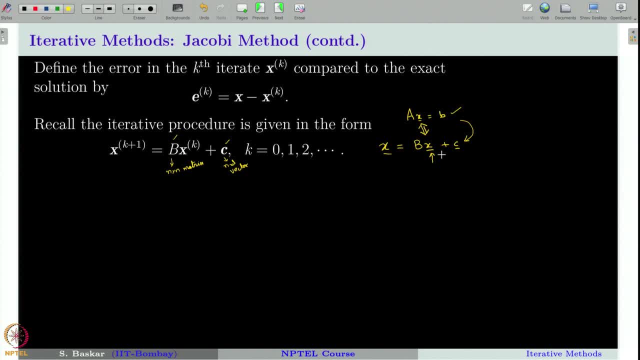 then we have plugged in a known quantity on the right hand side and got the corresponding vector and called that as the terms of the iterative sequence right. So therefore we also have this equation satisfied by the exact solution. therefore the error involved in the case. 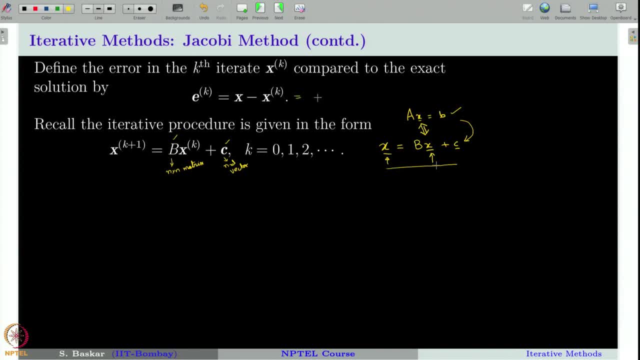 The eighth iteration can be written as b, x plus c, which I am replacing with this x and x k is replaced by its formula, which is given by b, x, k minus 1 plus c. right, Therefore you can get this as b, which is a matrix. therefore, you can write it as b into x minus x k minus. 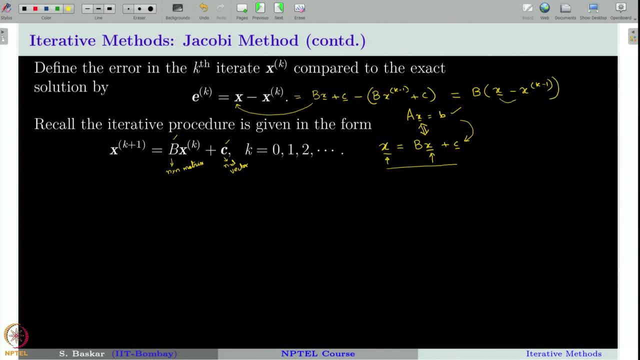 1 right. and this is again the definition of the error involved in the k minus first iteration right. Therefore you can write it as b e k minus 1 right. So therefore the error involved in kth iteration is nothing but b times error involved in the k minus. 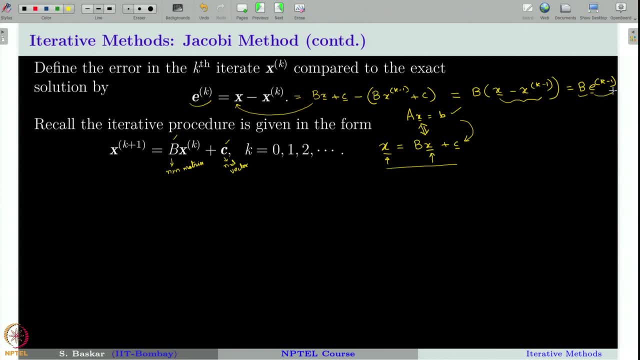 1 iteration. that is what I am writing. e k plus 1 is equal to b into e k. Now take the vector norm on both sides of this equation To get norm. e k plus 1 is equal to norm b e k. remember b e k is a vector. therefore, 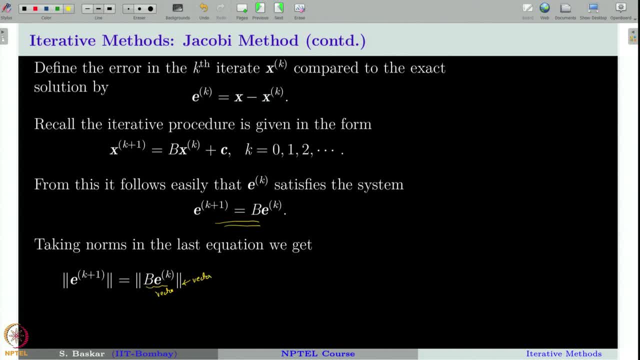 this is a vector norm right. Similarly, this is also a vector norm that we have taken. Since this is a general discussion, we are not restricting ourselves to any particular vector norm, like L 1 norm or L 2 norm or L e norm. 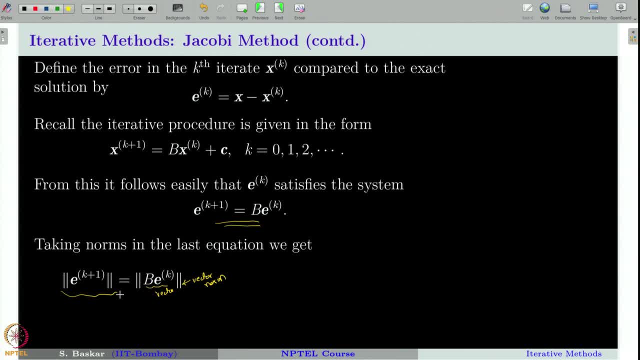 norm or L infinity norm. This discussion will go on with any choice of the vector norm. Now, if you recall, in one of the previous lectures we have discussed subordinate matrix norm. that is, matrix norm subordinate to a vector norm. right, What it is, you give me. 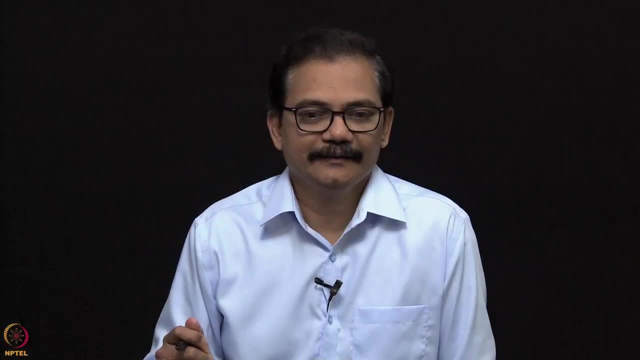 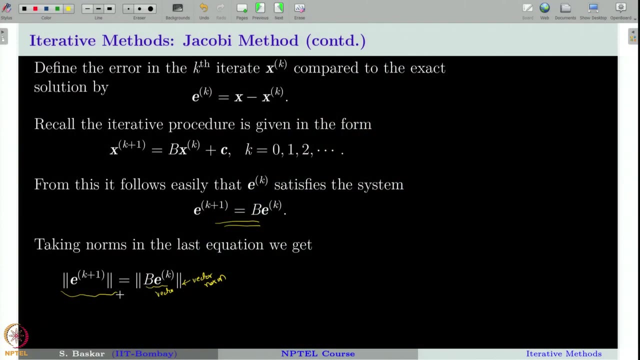 a vector norm. from there I will generate a matrix norm using that vector norm. right, Why we do that? because it satisfies three important properties that we have proved in one of the previous classes. Whenever you see an expression like this A into x kind of expression, you should immediately recall the property that this is less than or equal. 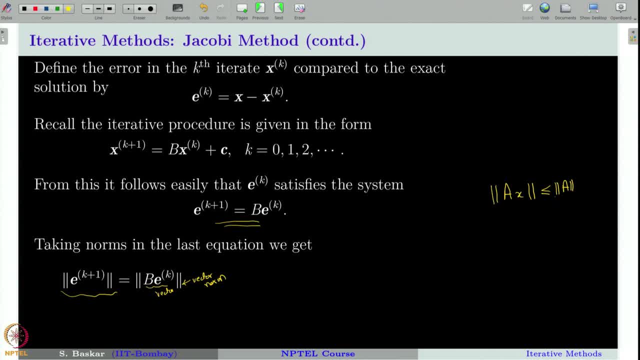 to norm A- This is the subordinate matrix norm- into norm x, which is a vector norm. Here also you see a similar expression here: B into E, where B is a matrix, E is a vector. Therefore this can be written as less than or equal to norm B, which is the subordinate. 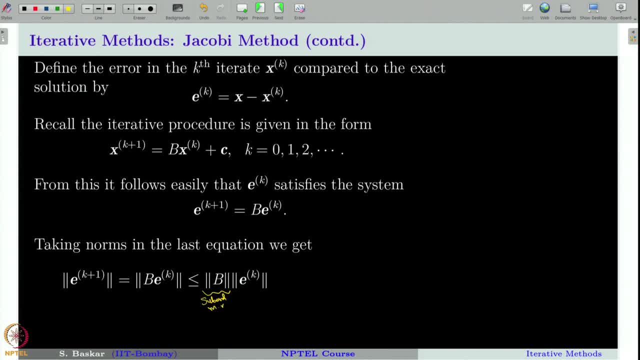 matrix norm and this is the vector norm. And now you see, this inequality holds for every k In particular. it also holds for E k. that is, you can write E k as norm B into norm E k minus 1.. Now if I apply that here, I will get: this is less than or equal to norm B. 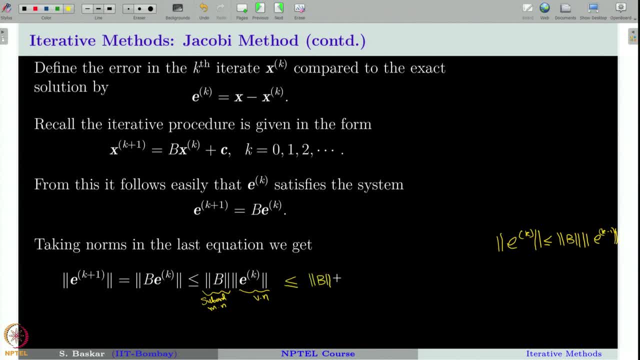 Now one more norm B will come from here and makes it norm B square into E k minus 1.. Again, you apply the same inequality for this term and that will give you norm B cube times E k minus 2.. So like that you can keep on going. 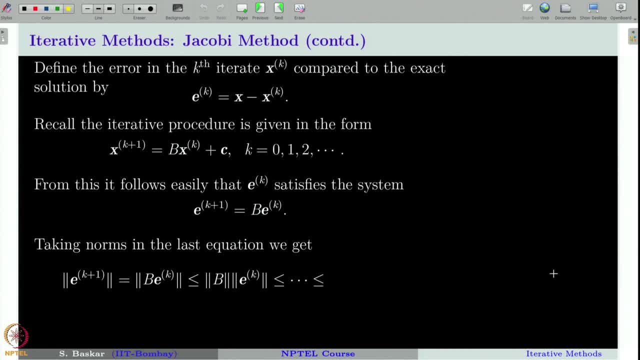 Thank you, up to E 0.. When you reach E 0 here, correspondingly we will get norm b to the power of k plus 1.. Now you see, this term is some finite number. Why? Because we have chosen x, naught arbitrarily. 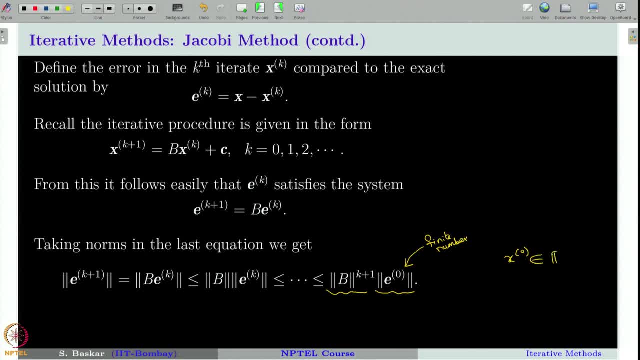 right, We will choose it in the space or n. Therefore, norm x minus x naught, which is precisely your E naught, is going to be surely some finite number. right Now, what is our interest? If you recall, our interest in this discussion is to see when. 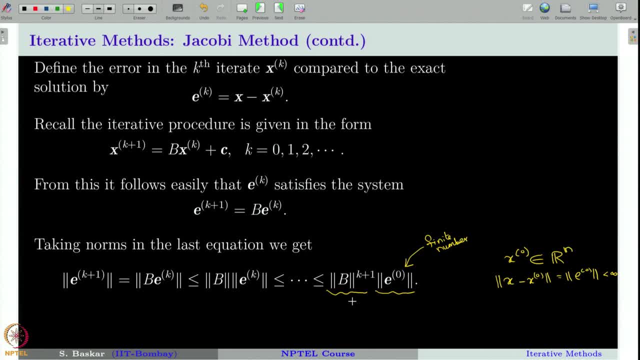 our Jacobi matrix, Jacobi method, that is, the iterative sequence generated by the Jacobi method, should converge, right? when will it converge? is the question. Equivalently, the question is to see when this term goes to 0 in some sense, right? Well, if this goes to 0, then x k goes to x, right? 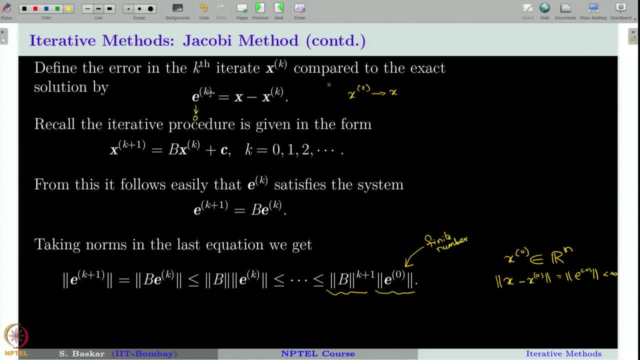 Therefore, our interest is to see when this term goes to 0. in some sense, for that we have taken a norm. It means we are trying to see this condition in the sense of a given norm, that is, we want this term to go to 0, right. 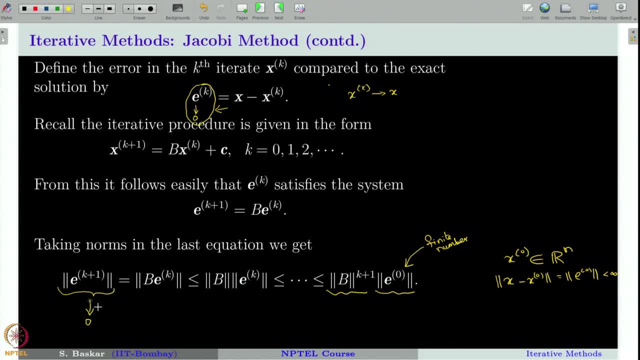 From this inequality. we can see that this happens when this term goes to 0, because this is already a fixed number. Therefore, this is already a fixed number. Therefore, we want this goes to 0 if this goes to 0. Why it is so? We know that the norm is always greater. 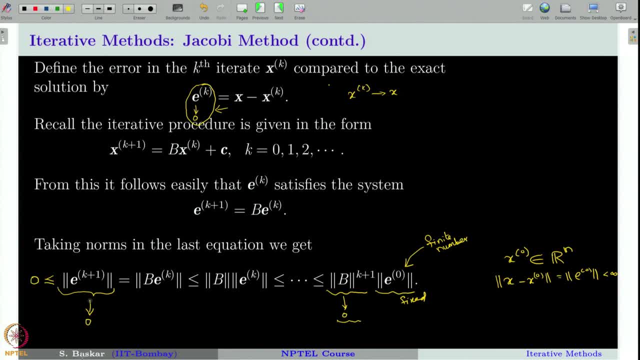 than or equal to 0.. Therefore, if this term goes to 0,, then you can apply the sandwich theorem for sequence to see that this is already 0, and if this goes to 0, then this will also go to 0. that is the idea. Now the question is when this term goes to 0,. when this term 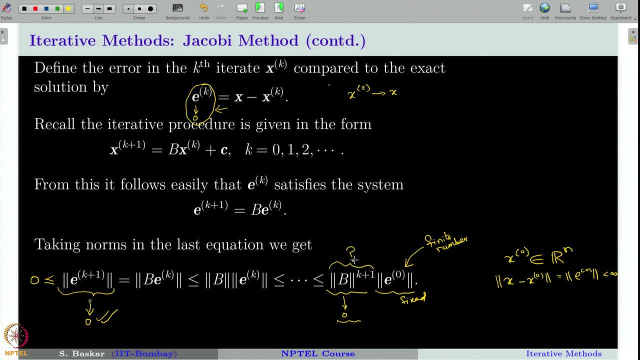 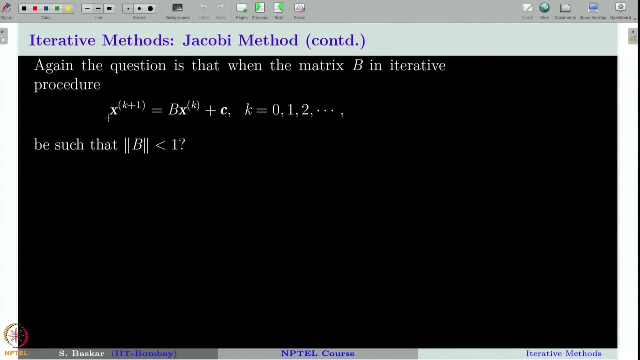 goes to 0.. Well, we can clearly see that this term goes to 0, as k tends to infinity if norm b is less than 1.. So, to summarize, we want this sequence to converge right. In order that this sequence should converge, we need E, k with respect to some given norm. 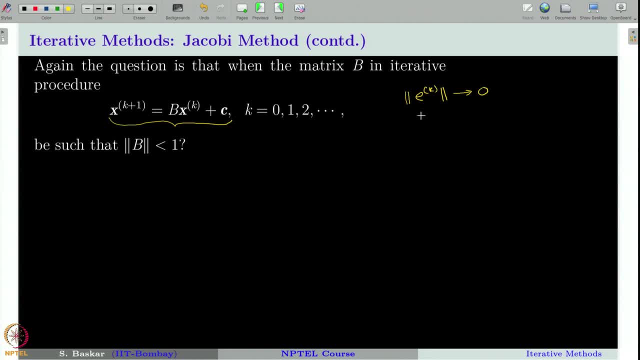 should converge to 0. We have just now seen that if norm b is less than 1, then the error will converge to 0 with respect to the vector norm. Remember, you choose a vector norm and you want E k to converge to 0 with respect to that vector norm. for that this Jacobi iterations matrix. 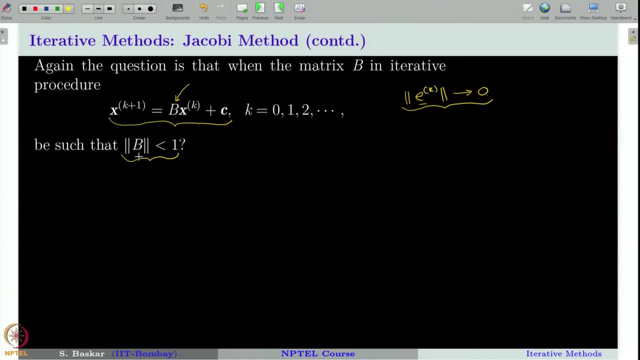 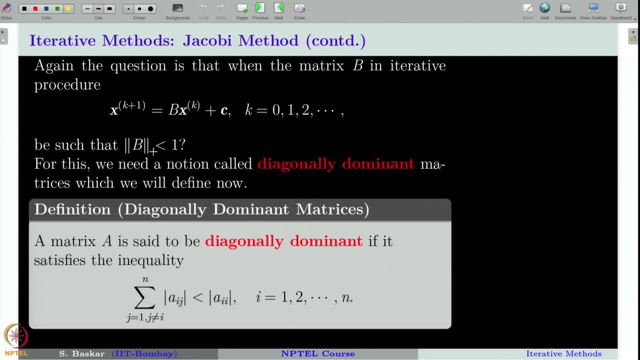 should have its corresponding norm, So its corresponding subordinate matrix norm to be less than 1. when can we say that a matrix is diagonally dominant? Suppose you have a matrix A which is given by a, I, j, where i varies from 1 to n and j varies from 1 to n. Say, for instance, you take a matrix, something, 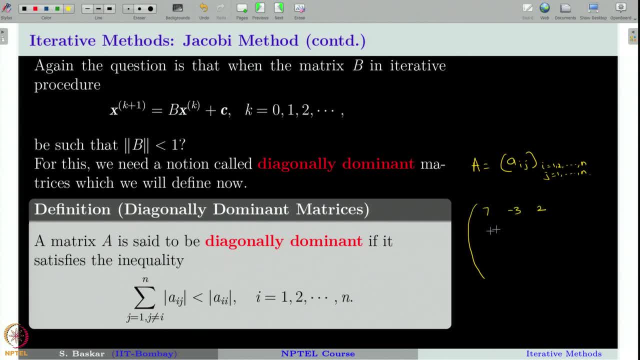 like 7 minus 3 and 2.. 0,, 2 and 5 and minus 1,, 1 and 3.. So to check whether this matrix is a diagonally dominant matrix or not, what you have to do is you take all the terms other than the diagonal term. 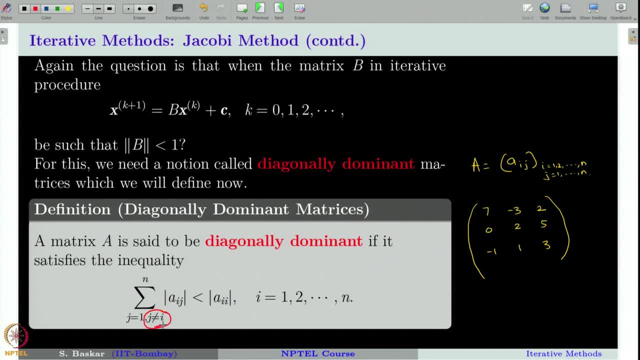 that is what we meant by saying j not equal to i Remember you fix a i, for instance, you fix, say first row, and take all the non-diagonal elements, take their absolute value and then sum them up. that is what the left hand side says In this example. it is nothing but 3. 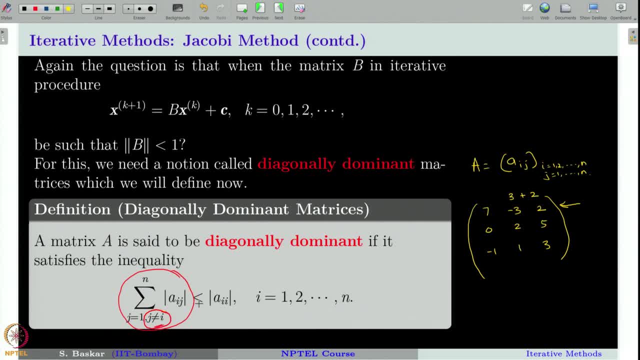 plus 2, and that should be less than 3 plus 2.. So the absolute value of the diagonal term, that is, this, should be less than the diagonal term, that is 7 in the first row. Similarly, you take the second row. you see that the non-diagonal 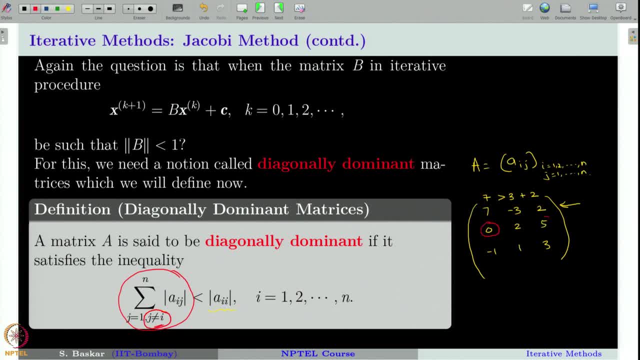 elements are 0 and 5.. Therefore, 0 plus 5 should be less than the diagonal element, which is 2.. So this is not happening. therefore, this matrix is not a diagonally dominant matrix, because this should happen for all the rows. So you remove the diagonal element and sum. 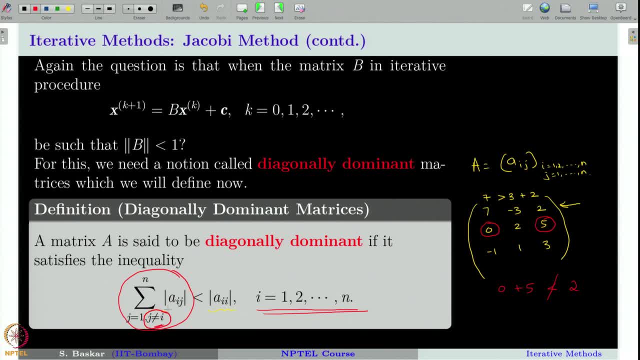 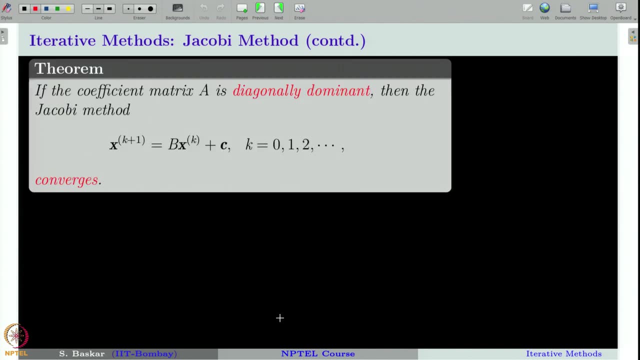 all the non-diagonal elements of a row with their absolute value and then check whether this inequality is satisfied. Then we call the matrix A as diagonally dominant. Now our convergence theorem says that if the coefficient matrix A is diagonally dominant, then the Jacobi method converges. It means 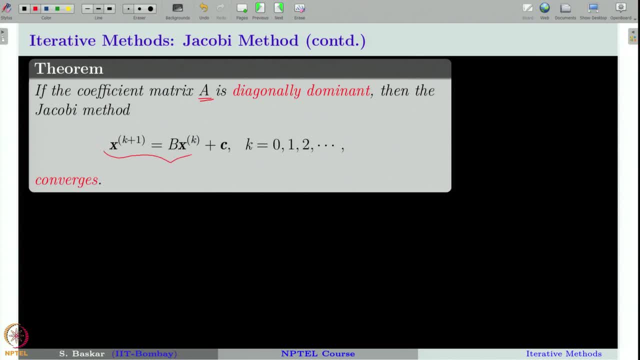 the iterative sequence given by this expression converges. Now the idea is to use the condition that the coefficient matrix is diagonally dominant And prove that norm B is less than 1. that is the idea of the proof of this theorem. We will present this theorem by choosing some particular norm, which is the L infinity norm. 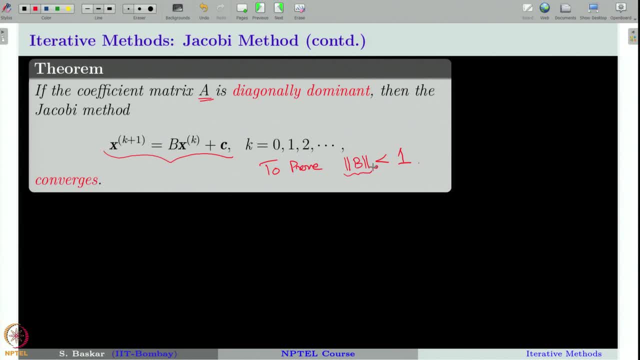 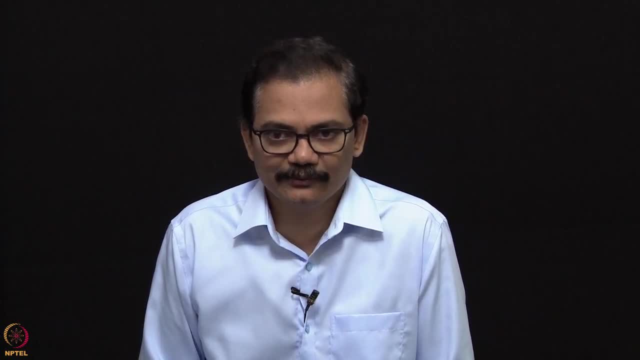 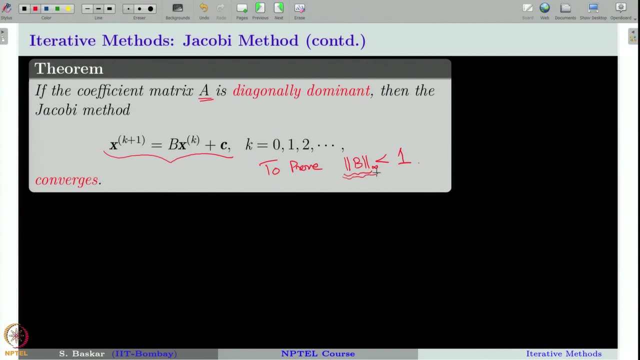 because in that way the proof goes more nicely and it is easy to understand. Therefore, in the proof of this theorem we will Consider only L infinity norm to compute the quantity norm B and see how it goes. The theorem says that if A is diagonally dominant, then the Jacobi iterative matrix, this is called. 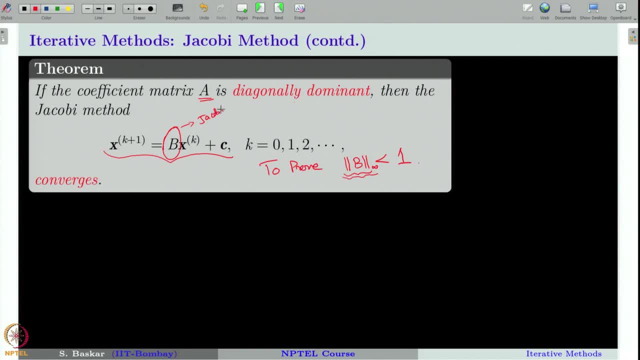 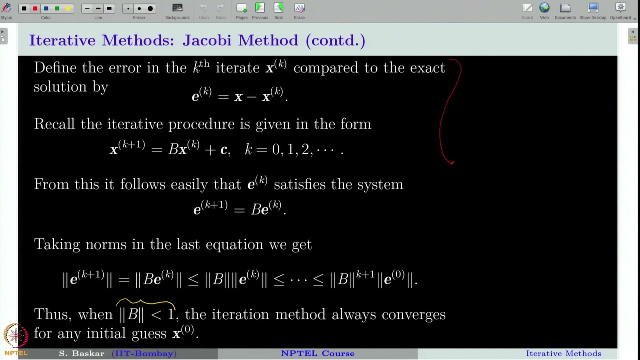 the Jacobi iterative matrix, We will have its subordinate matrix norm to be less than 1.. Well, the proof of this theorem is more or less similar to what we have shown here. Only thing is the same: derivation we will do coordinate wise in order to see how the diagonally dominance of the matrix 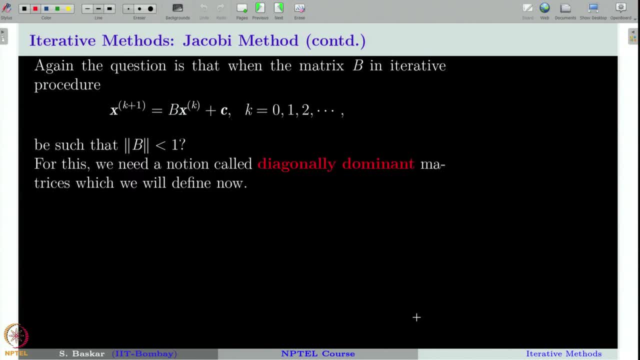 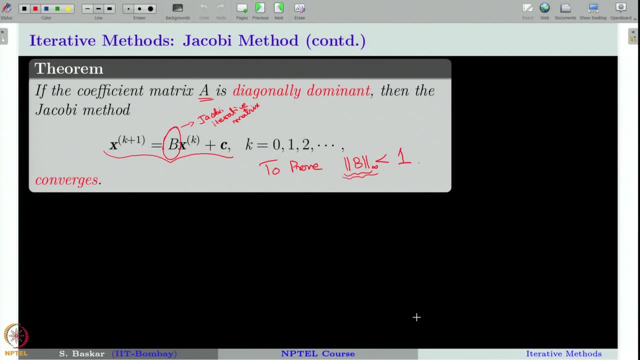 A is going to make this quantity norm B to be less than 1.. To very clearly see this, we will do the same computation, coordinate wise. Remember this equation is given like this for each coordinate: How it is. So what we are doing is suppose: 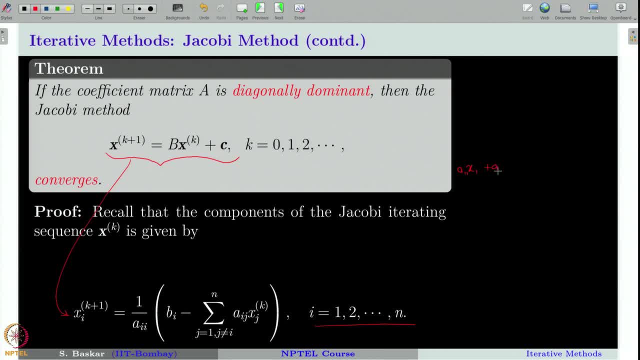 you have A 1 x 1 plus A 1, 2 x 2 plus A 1 3 x 3, equal to B 1. If you take then what you are doing in the Jacobi method, you are keeping the diagonal element, Since this is: 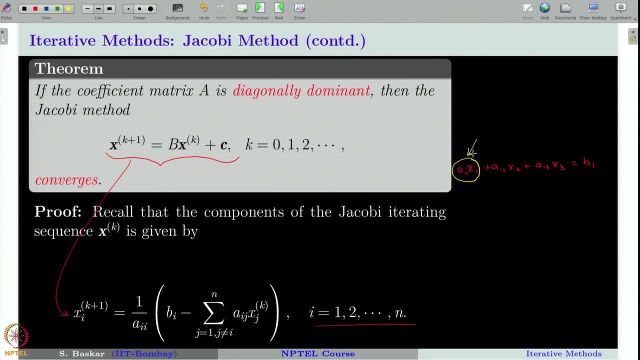 the first equation of your system. the diagonal element is the first term. You are keeping that on the left hand side and then taking all the other elements, that is, A 1, 2 x 2 plus A 1, 3 x 3 on the left hand side. 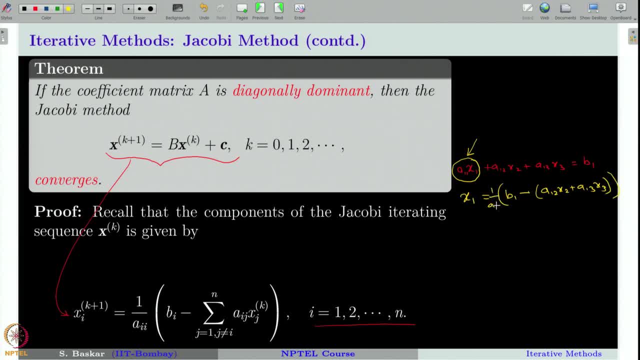 And finally, dividing both sides by 1, by A 1- 1.. That is what I am writing here. The ith equation can be written as: x i is equal to. I am dividing by the diagonal element A i. i, then keeping B- i as it is all the non-diagonal. 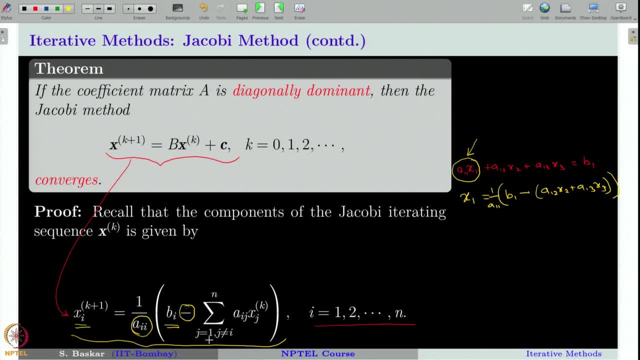 elements are taken on the right hand side. Therefore, you have a minus here and then the summation. This summation, remember it- will exclude the diagonal element because it was not taken to the right hand side. That is why we have written j not equal to i and 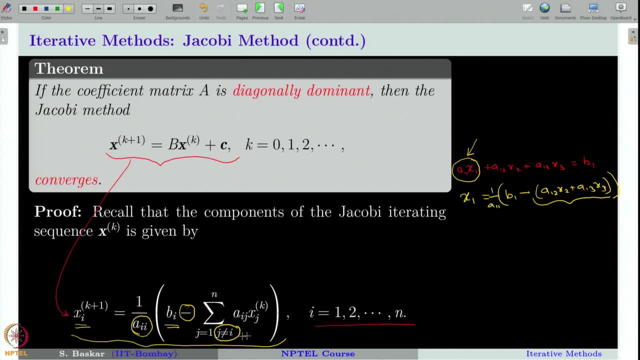 this is for one typical equation, that is, the ith equation, and that i will run from 1 to n. This is precisely what the Jacobi method is, Remember. the same equation also holds for the exact solution. That is what we remarked, that is, x. i is equal to A: 1 x 2 x 3 x 2 x 3. 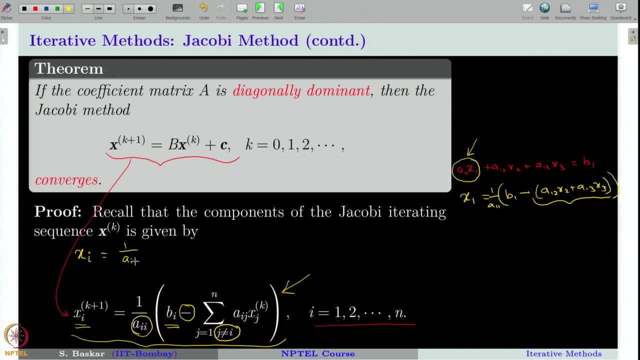 i can be written as 1 by A i i into B i minus sigma, j, equal to 1 to n j, not equal to i. A i j into x, j, k. Now if you subtract these two- x i minus x, i k plus 1, that will give: 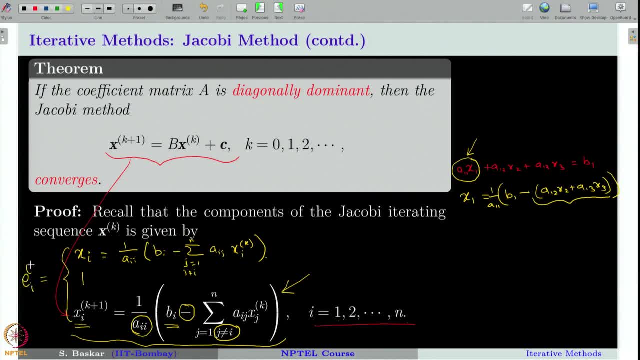 you the ith component of the vector error. When you subtract these two, this gets cancelled. Similarly, you will have here the coefficient A. i, j will remain, and then you will have x, j, k. There is no k here. This is exact solution. 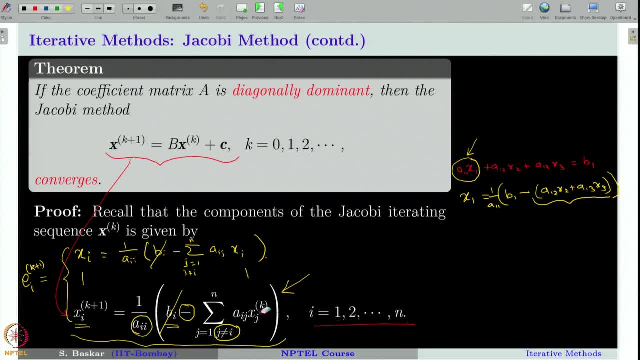 Therefore x j minus x j k will come. That will give us E j k. Therefore, you will have E j k plus 1 is equal to minus, because this minus is here sigma j equal to 1 to n j, not equal to i A. i j divided by this diagonal. 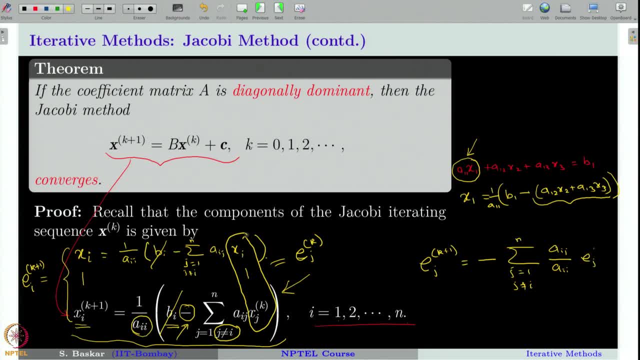 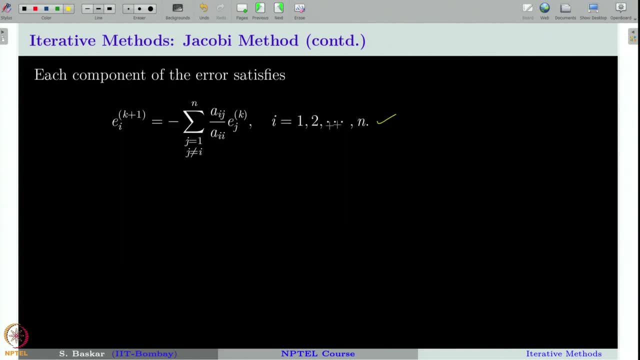 element A, i, i into E, j, k. So that is what we are having here and this should hold for each equation, that is, for: i is equal to 1, 2 up to n. So the corresponding error involved in the Jacobi iteration at the k plus 1th iteration is given by this expression. Now 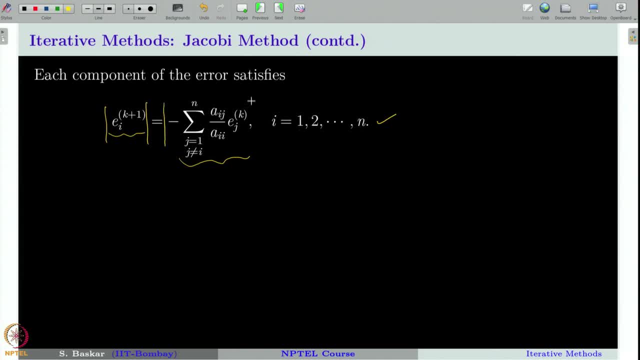 you take the modulus on both sides and then you take the modulus inside the summation that will give you this to be less than or equal to norm of this, into norm of this. There is a plus sign here. Now what happens is: remember your E k vector is nothing but the. 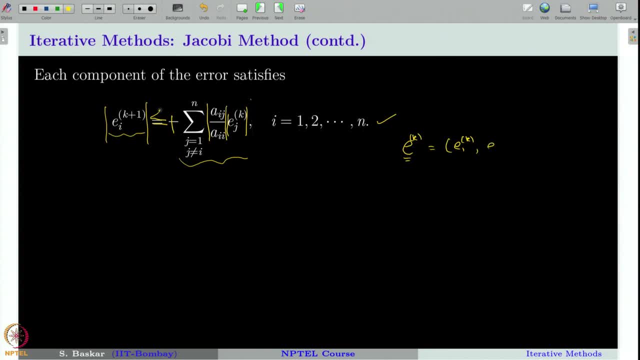 E 1 k, E 2 k and so on up to E n k. Now what is the infinite norm of E k? It is nothing but maximum over all mod E, i k's or may be E j. I will put here. J varies from 1 to n. 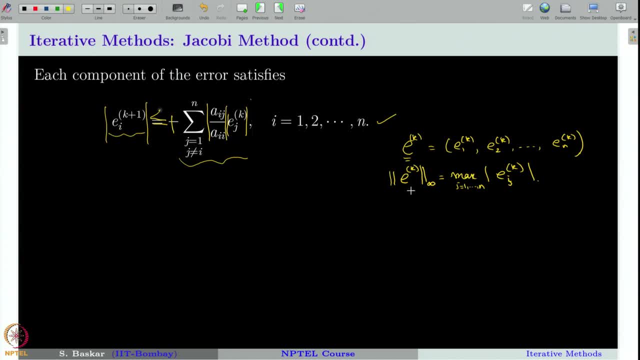 So let us say, in each of these terms: what if I replace each of this term by its infinite norm? Then I can say that this is further, less than or equal to sigma A, i, j, divided by A, i, i into norm E, k, infinity, because I am replacing each term in this sum by its 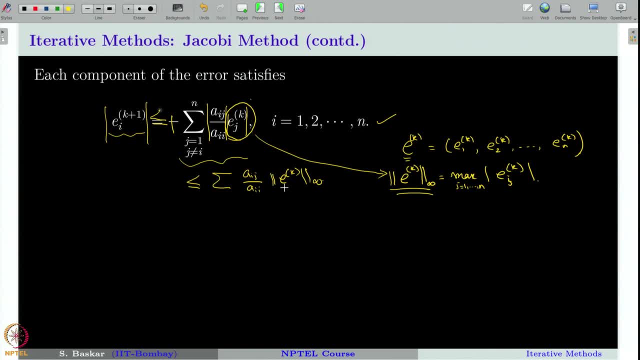 maximum value. Therefore, that will give me, That will give me something value bigger than this. Therefore, I will have this inequality. Now, you see, this inequality still involves this term. Let us see how to dominate this term. You see, for each i, you have this number, i is equal to 1, you have a number like this: 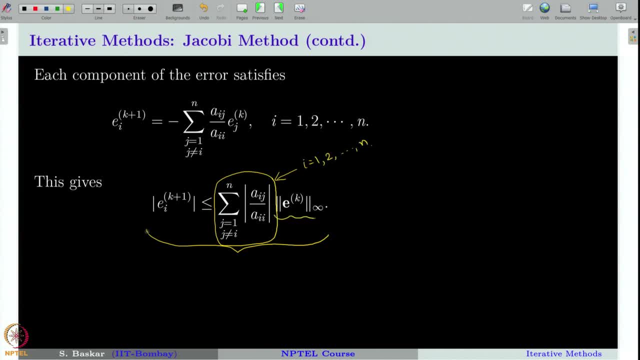 2, and so on up to n. This is common for all these i's because it does not depend on i, as well as it does not depend on j. Therefore, it will also come out of this summation and you have this. 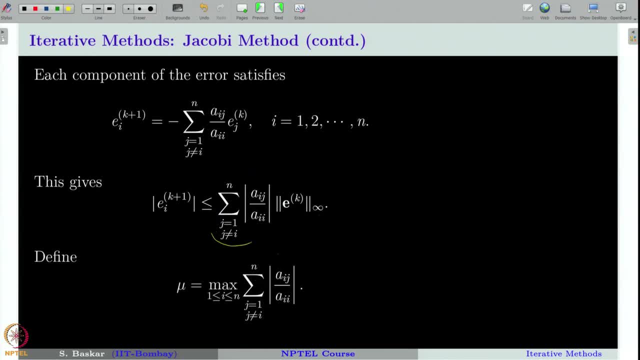 Now take the maximum over all these numbers. Take maximum over all these numbers and call this as mu. Then you can say that this is further, less than or equal to mu times norm E, k, infinity. So that is what we are getting here. mod E, i, k plus 1 is less than or equal. 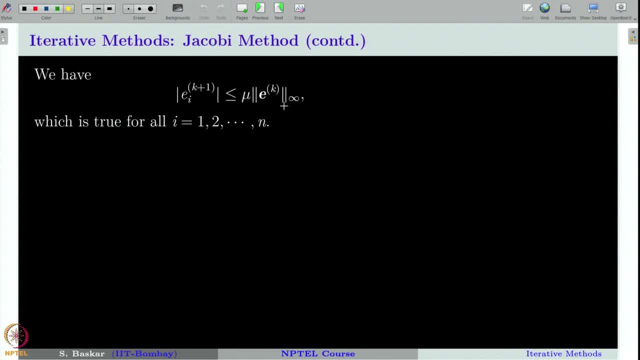 to mu times, infinite norm of E, k, and this happens for all i, equal to 1, 2, up to n. Remember, the right hand side is independent of i, whereas the left hand side depends on i, and this inequality, this inequality holds for all i. Therefore, you take, suppose you take, this quantity which 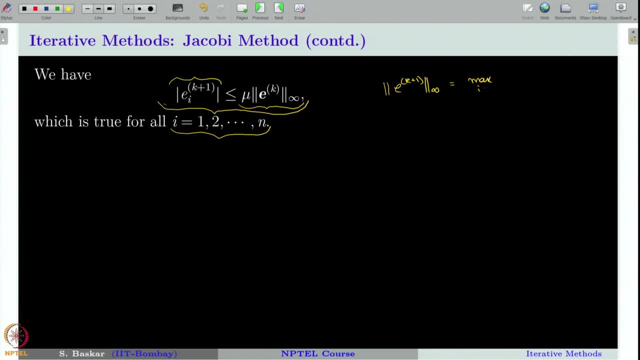 is nothing but maximum over all i, equal to 1,, 2, n, such that norm E, i k plus 1.. So this maximum will achieve at some index between 1 and n, right? So therefore this inequality will hold for that index also, because this holds for all i. Therefore it will also hold. 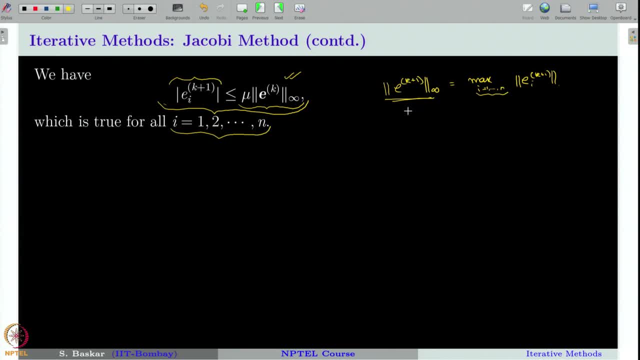 for that index at which the maximum norm is achieved. Therefore, you can write with respect to that maximum norm also. that is, you can replace this by the maximum norm, because it holds for all i. Therefore it will hold for that coordinate at which the maximum norm. 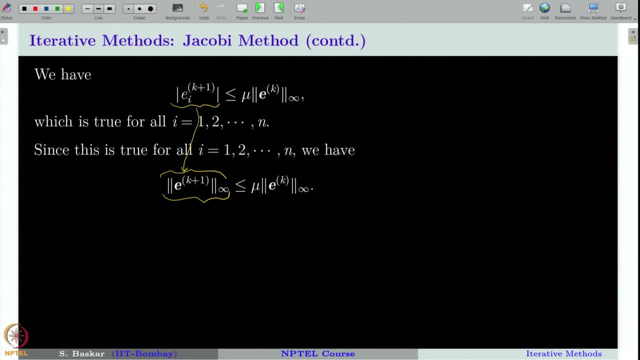 is achieved, and that is less than or equal to mu times, E, k, infinity. Now you see, finally we got this inequality, and this is again a recursive inequality, in the sense that you can apply this inequality to this term, just like what we did in the 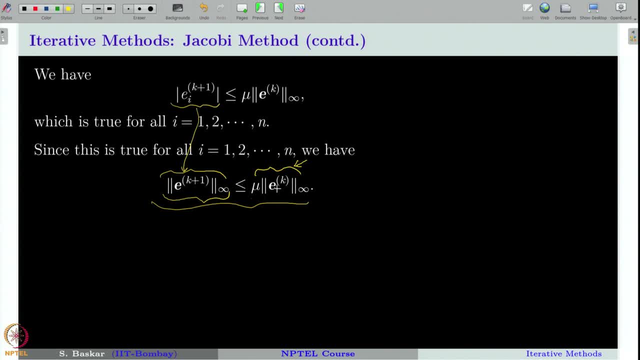 previous slide. You can apply this inequality to this and that will give you mu into mu times norm E k K minus 1, and that will actually give us mu square norm E k minus 1, infinity. Again, you do the same idea. You can say that this is less than or equal to mu cube into norm. 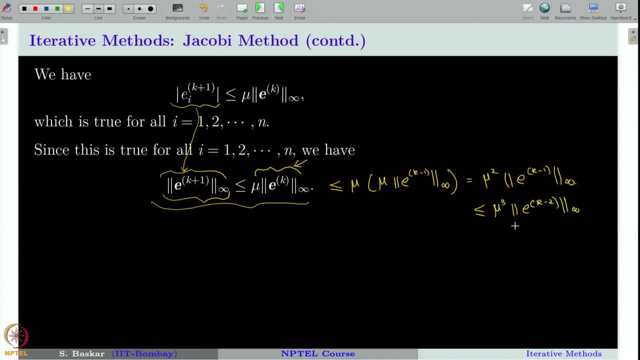 E k minus 2 infinity and so on. You can go until where you can go up to E 0 here and correspondingly that will give you as norm E k plus 1 infinite norm is less than or equal to mu k plus 1 times infinite. 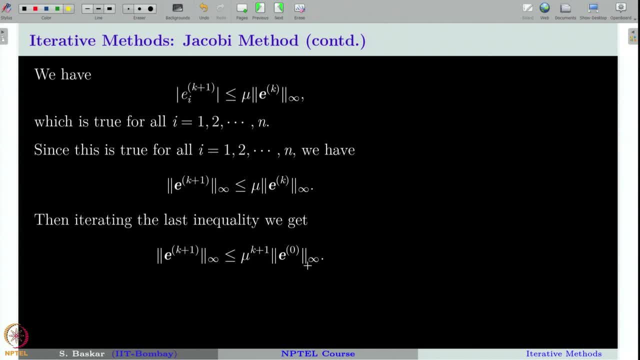 norm of E 0.. Now, if you recall, in tutorial 1, we have solved a problem where we have seen that if your sequence x- n is such that x n minus L is less than or equal to mu k x n into x 0 minus L, If that is so, then you can say that this sequence x- n converges. 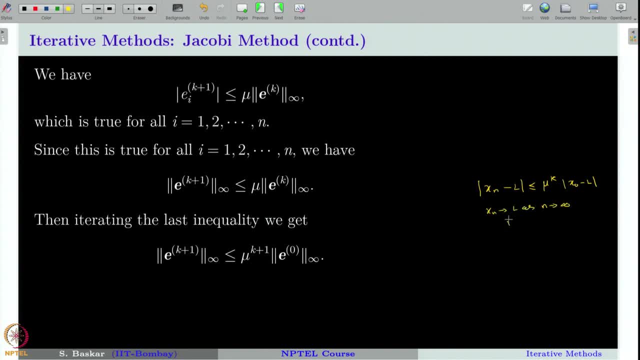 to L, as n tends to infinity if mu is less than 1.. This is n here. Now we have the same kind of inequality here. Therefore, you can see that here we have this inequality and that if mu is less than 1, then of course this goes to 0, as k tends to infinity. You 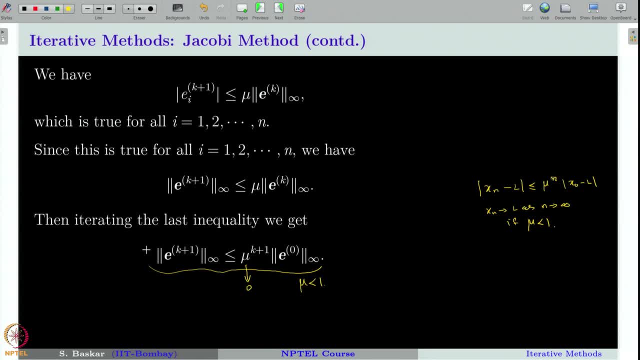 can also see this result using the sandwich theorem, because this is always greater than equal to 0, and so if this goes to 0, this is a fixed number, right? Therefore, this will also goes to 0 as k tends to infinity, right? So that is what we get. Therefore, all we 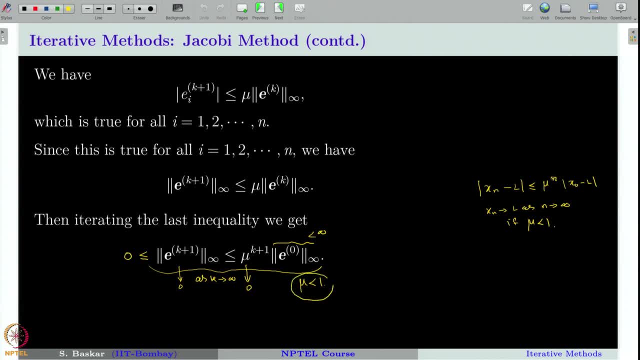 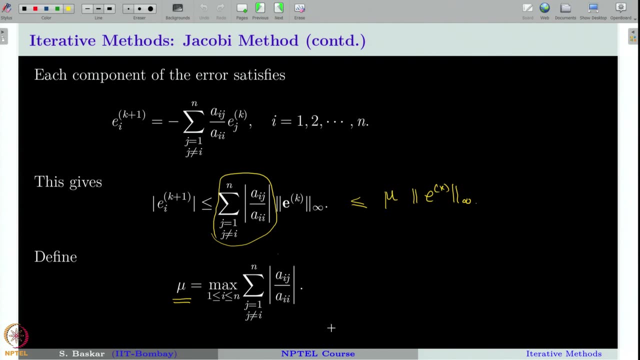 need is to see whether this mu is less than 1 or not. In fact, from the way mu is defined, you can see that this is true if A is a diagonally dominant matrix. So if A is diagonally dominant, then A, i, i will always be greater than sigma j equal. 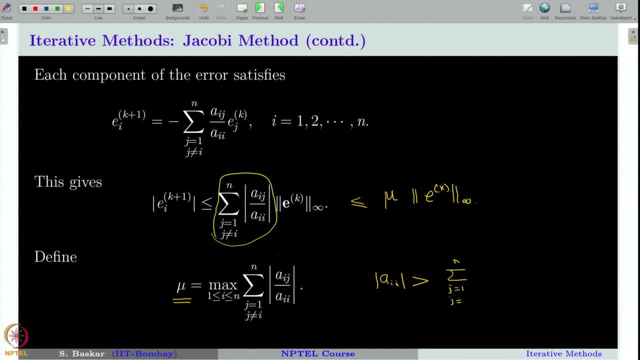 to 1 to n. removing the diagonal term that is, j, is not equal to i, right times mod A, i, j. Therefore, all these terms, all these terms are less than 1 and now you are taking maximum of all these terms. 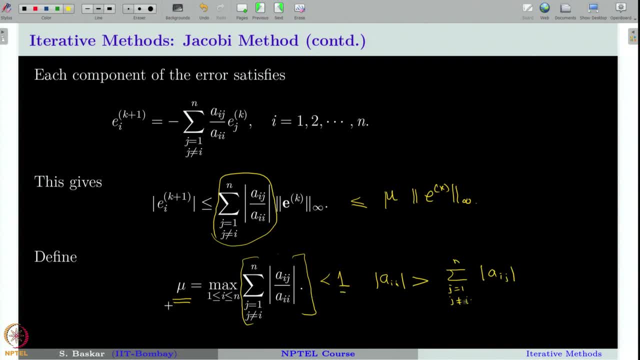 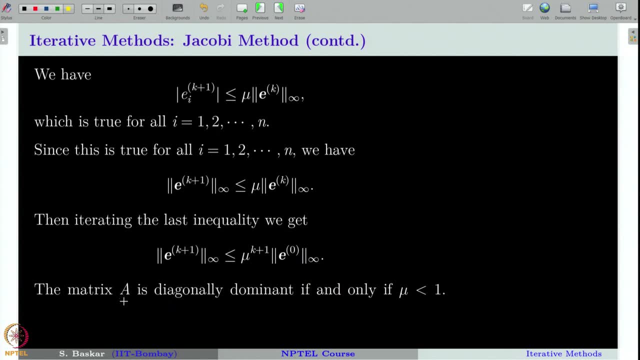 all numbers which are less than 1. therefore, mu will also be less than 1.. So this is what precisely we wanted to show: that if A is diagonally dominant, then the Jacobi sequence converges, that is, x, k converges to x as k tends to infinity is what to prove. 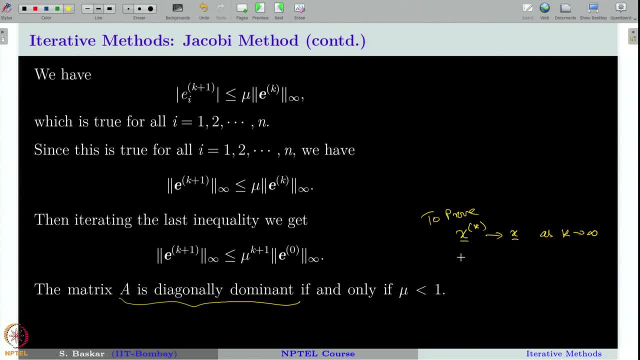 What we did is we just took the infinite norm and try to prove this. This is equivalent to saying that E, k, with respect to infinite norm, tends to 0, as k tends to infinity. By going into coordinate wise, we have seen that the required term, that is, infinite norm of 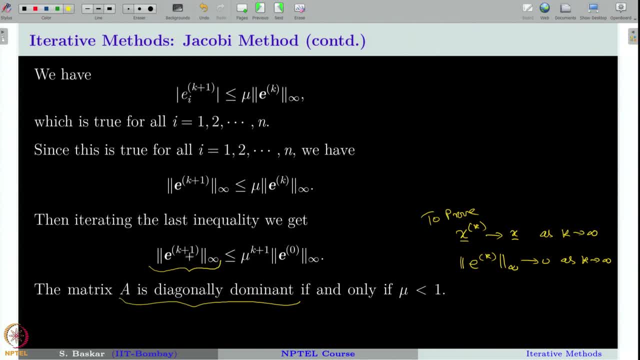 E k will. here we did with one index more E k plus 1 is less than or equal to this quantity times the infinite norm of E 0, and by imposing the condition that A is diagonally dominant, we saw that mu is less than 1.. Therefore, 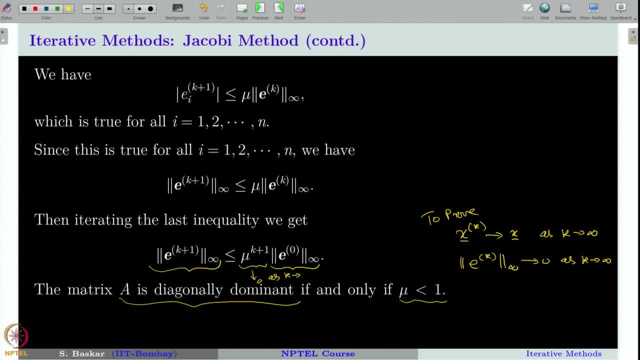 this goes to 0 as k tends to infinity and therefore by sandwich theorem we can see that this goes to 0 as k tends to infinity. So that completes the convergence proof for Jacobi method. Remember that this theorem gives only the sufficient condition for the 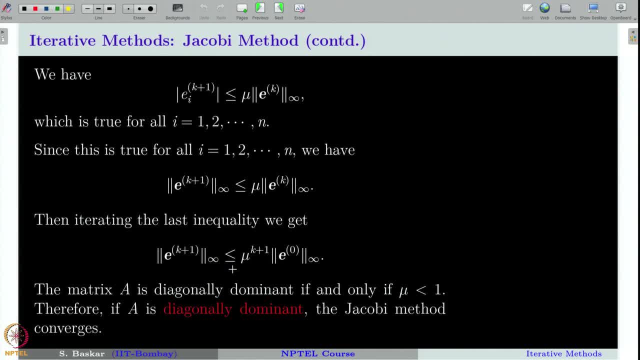 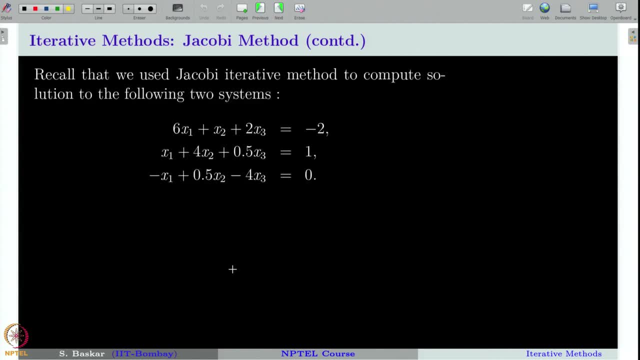 convergence of the Jacobi method. With this, let us go to the examples that we have discussed. in the last class, If you remember, we considered two examples. In the first example we took this system and we have seen that the Jacobi iteration tends to infinity. So this is the 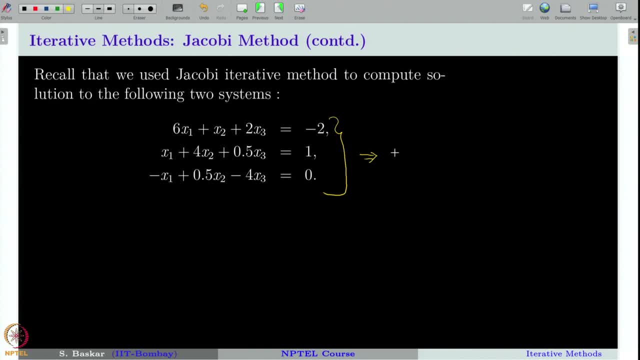 case where we go closer and closer to the exact solution as we go on computing the iterations. On the other hand, the second example that we took, where we took this system- this tend to go away from the exact solution x. That is what we have seen in the last class. So 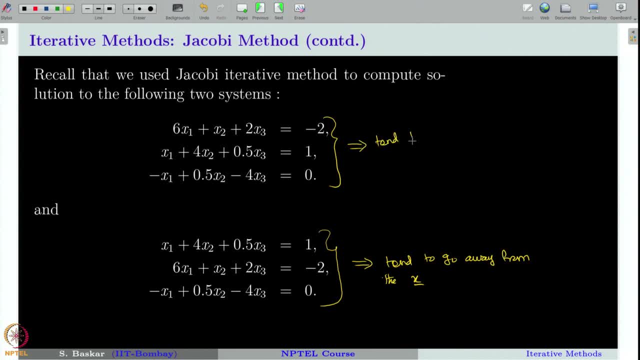 it is more clear for us why this system was behaving well in terms of the Jacobi iteration, because this system is diagonally dominant, Whereas this system is not diagonally dominant. So that does not mean that the Jacobi iteration should diverge, because our theorem says only: 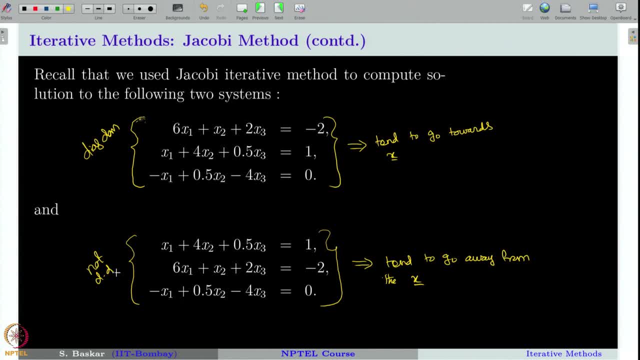 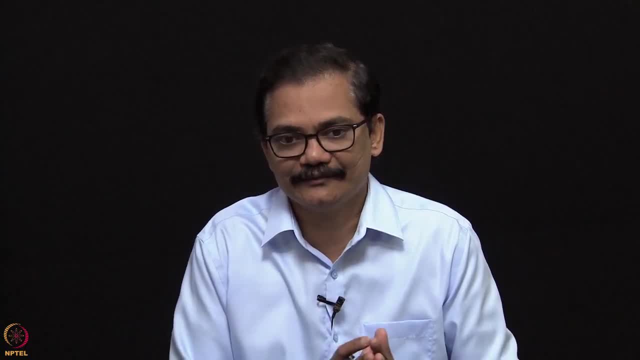 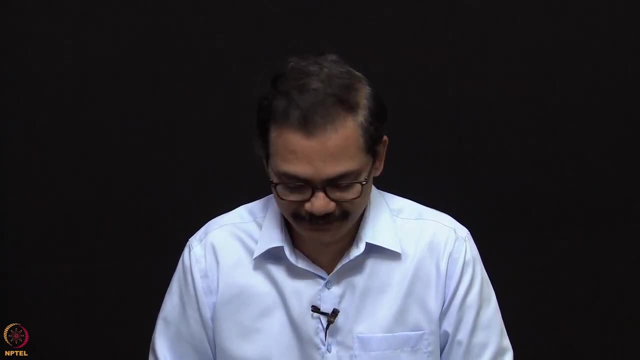 that the diagonal dominance of A implies convergence. If the matrix is not diagonally dominant, our theorem simply does not say anything. In other words, what we proved is only the sufficient condition for the convergence of the Jacobi method. Therefore, our theorem, 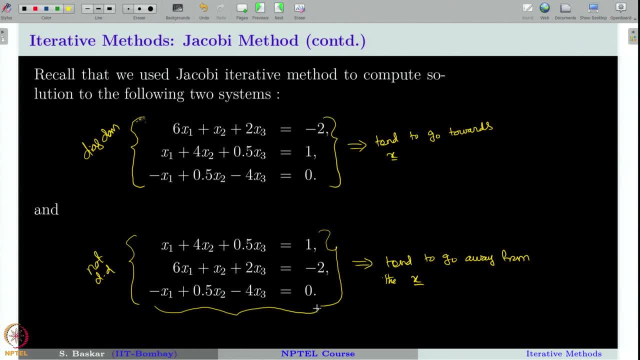 is simply silent for this system, because this system is not diagonally dominant. Numerically, we have seen, at least to the terms that we have computed, those terms of the sequence were going away from the exact solution. In fact, we can also get a necessary and sufficient